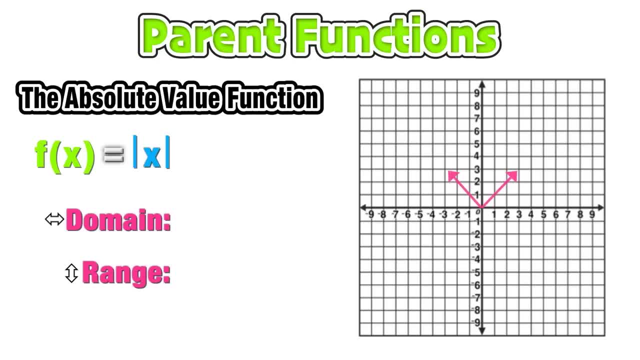 Our next parent function is the absolute value function. f of x equals the absolute value of x. We know that the absolute value is always positive, positive. that helps us to understand why this parent function remains above the x-axis and why the domain is negative: infinity to positive infinity, but the range starts at 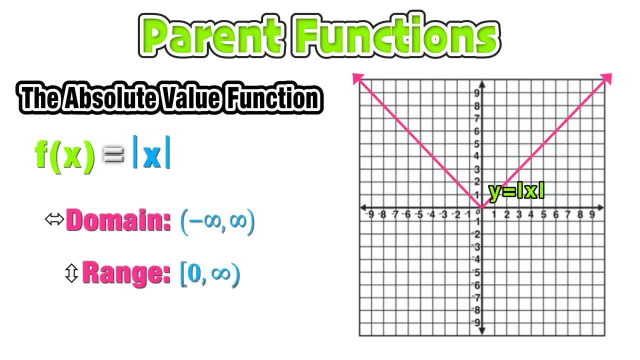 zero and moves up to positive infinity, but again, is never negative. Let's see what happens if we take this function and shift it to the left 5 units and then down 4 units. We can see that the parent function was transformed and moved to a new location. and we can also 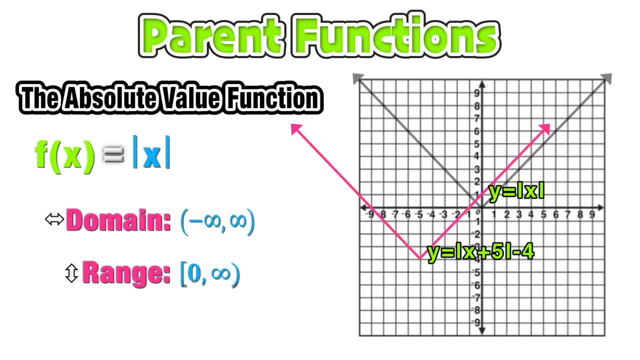 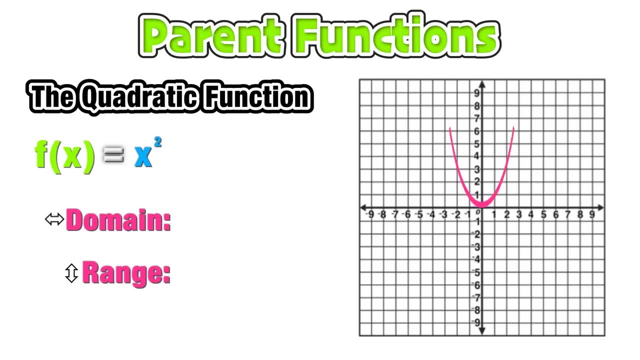 see how this new equation reflects that transformation. For this particular shift, we can see how the domain remained the same, but the range has to be adjusted. Now, instead of zero to infinity we have negative and 4 to infinity. The next parent function is the quadratic function. f of x equals x squared. 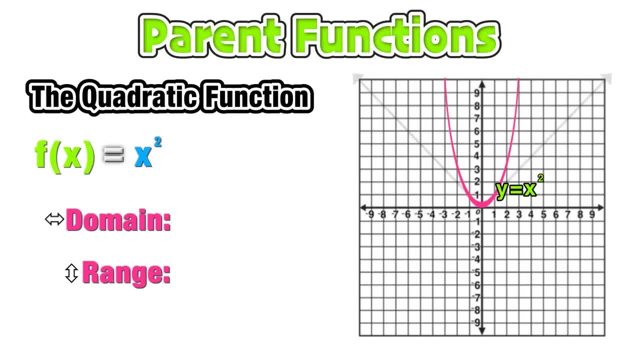 This parabola should look very familiar to us. If we compare it to the absolute value function, we can clearly see that it has the same domain and range, The domain being negative infinity to positive infinity and the range being from zero to infinity. 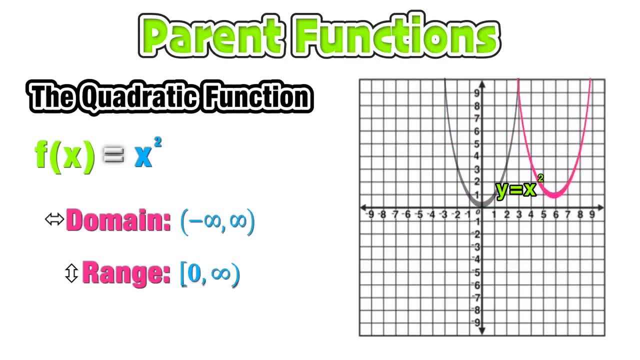 Let's go ahead and transform this function by shifting it to the right 6 units and then up 3 units. This new equation reflects the transformation on the parent function. y equals x squared, and we can see how the domain would stay the same, but the range would need to be adjusted. 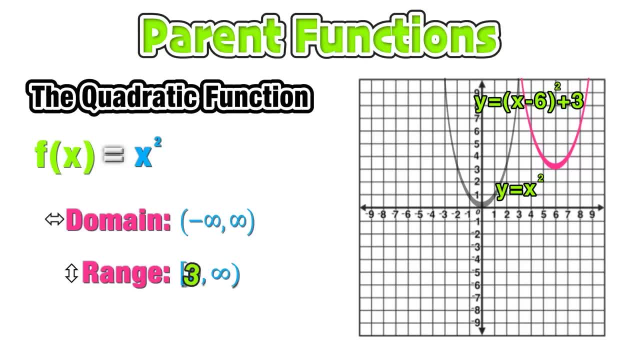 from zero to infinity, to 3 to infinity. That's it. Thanks for watching. The next parent function is the square root function. f of x equals the square root of x. This function has both a domain and range of from zero to positive infinity. 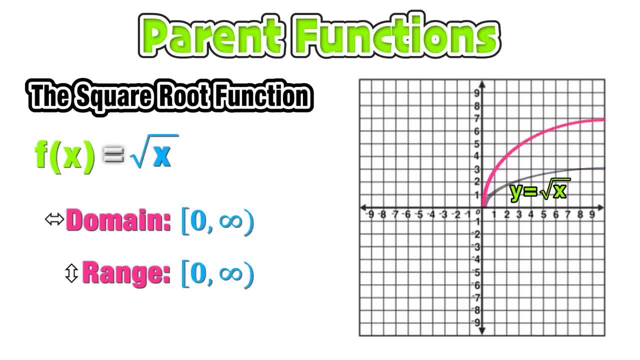 Now, if we were to multiply this parent function by a factor of 3,, we would have a new graph to represent. y equals 3 times the square root of x, but we can still see that the domain and range would remain the same.